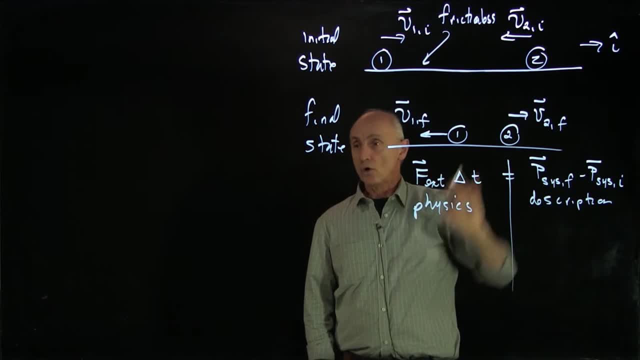 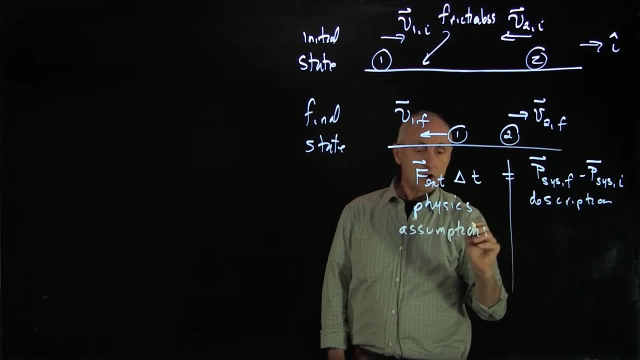 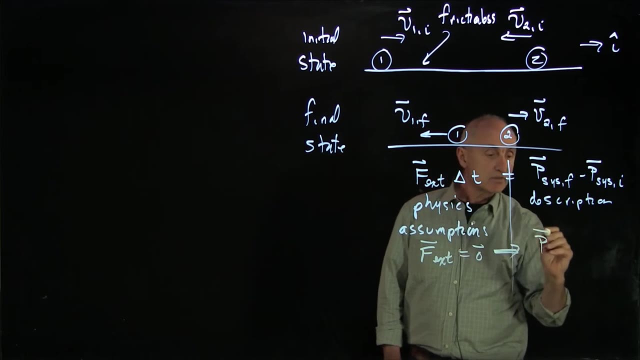 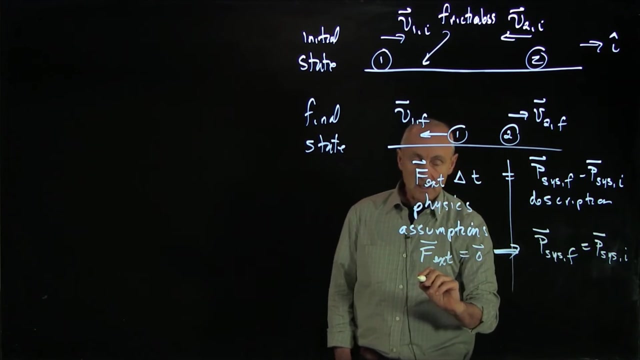 in fact, is frictionless and will ignore all air resistance. And so, by our assumptions that there are no f, external is 0. And therefore the momentum of the system remains constant. So here our statement is: many people call this conservation of momentum. 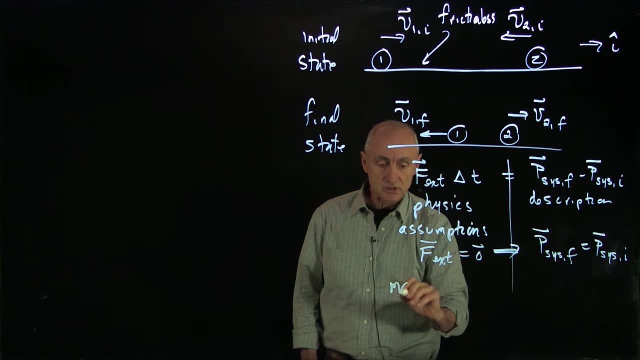 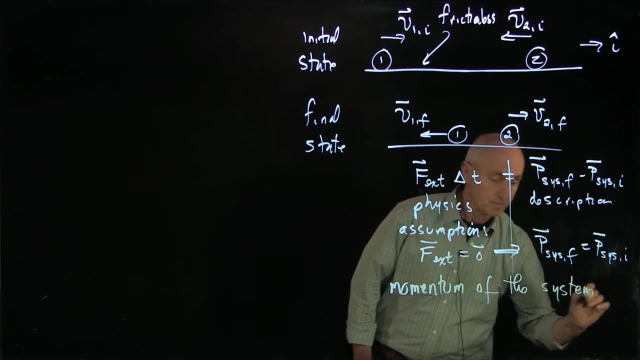 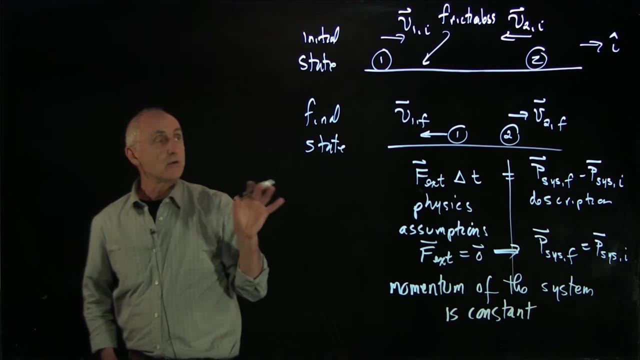 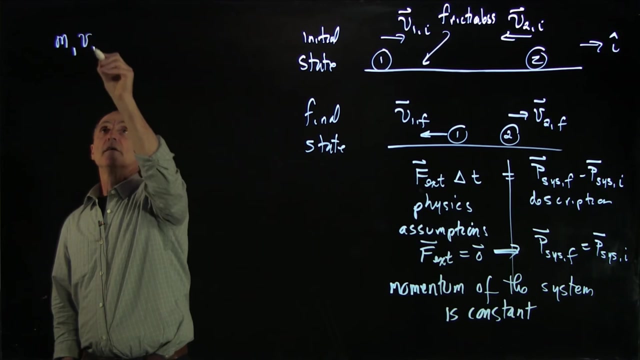 But we're saying in this example, based on our assumptions, that the momentum of the system is constant. Now, how do we actually write that down? Well, let's now write it first as vector expressions. So we have the initial momentum v1 of the system, m1, m2, v2. 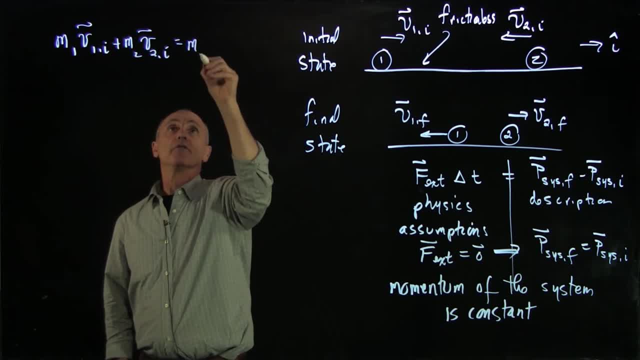 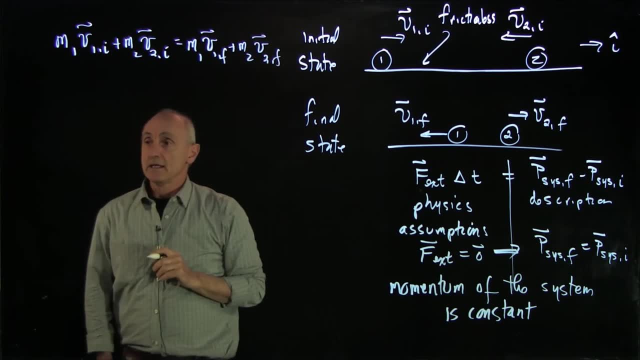 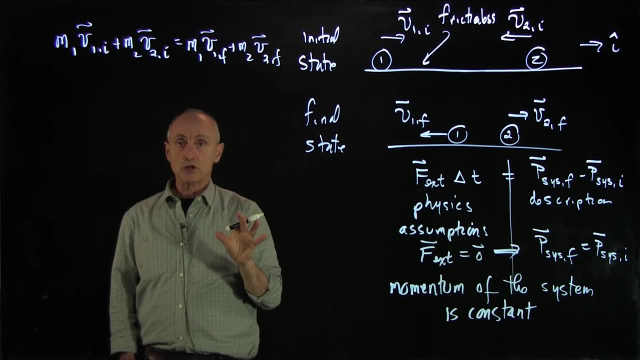 initial is equal to the final momentum, The final momentum of the system: v1, final, plus m2, v2, final. Now how do we represent these equations? Well, you could treat them as vectors, if you wanted, But what we're going to do is express them as components. 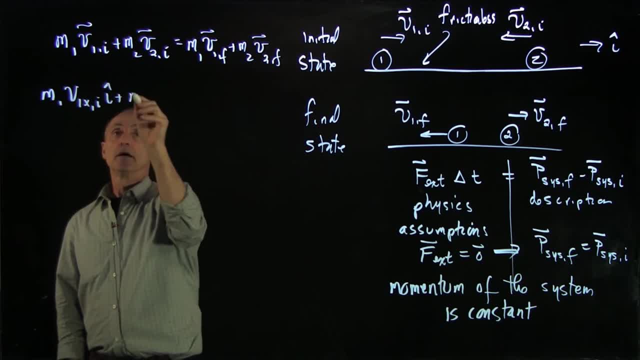 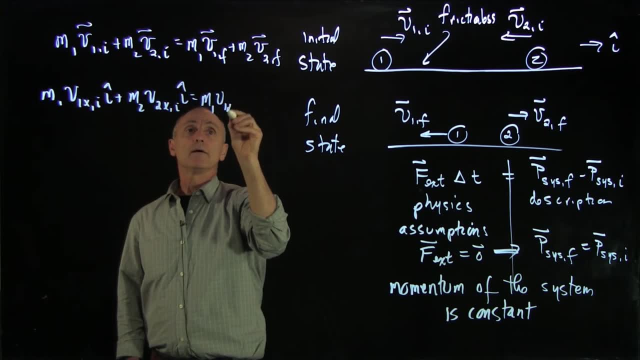 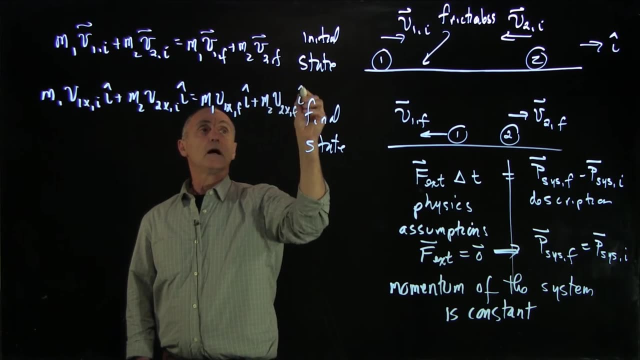 So if we wrote this as components, we would have m1, vx- initial i hat, plus m2, v2x- initial i hat. So this is m1, v1x- final i hat, plus m2, v2x- final i hat. 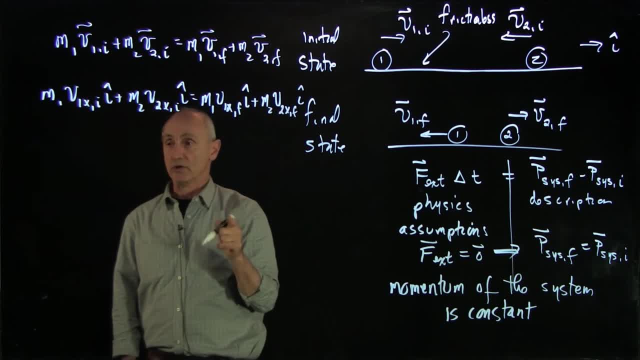 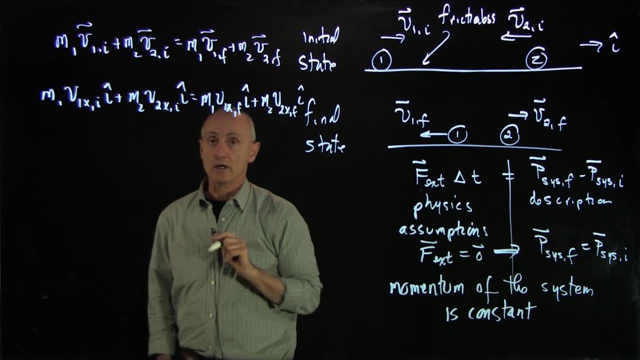 So that's the vector expression expressed in terms of components. The advantage of this is that we really don't know the signs of these two final components, That's, our target quantities, But we could just write this equation instead of writing it as a vector equation. 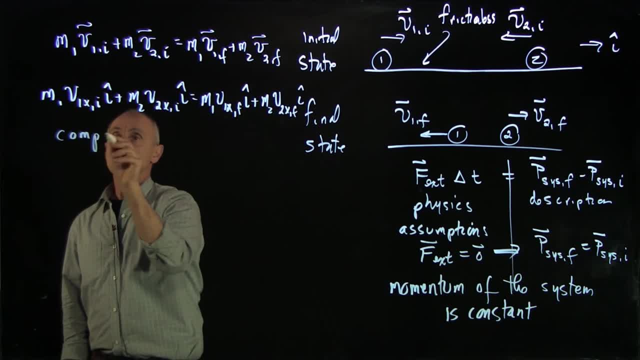 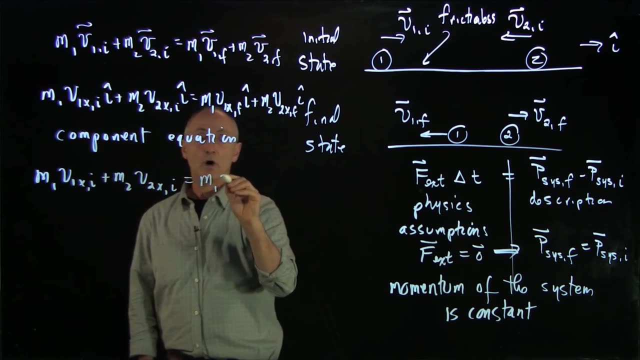 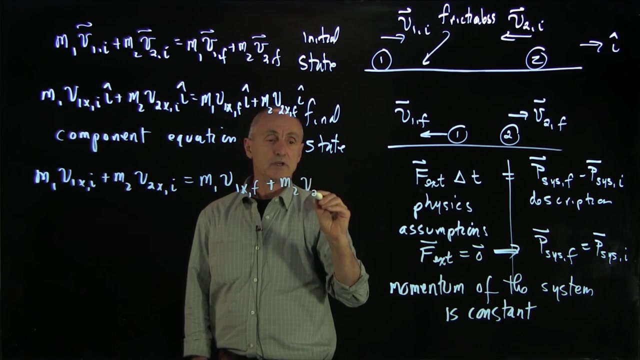 let's just now write this as a component Equation And when we write this equation in terms of components, we have m1, v1x initial plus m2, v2x initial equals m1, v1x final plus m2, v2x final.